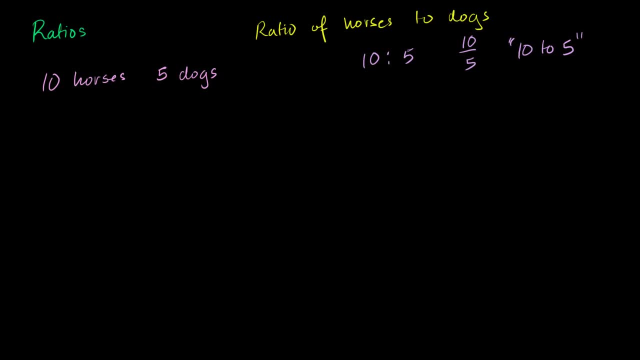 And the thing I write first, or the thing that I write on top, is the number of horses. So this is the number of horses right there. That's the number of horses, And that's all the number of horses. If I want to talk about the number of dogs, this is the 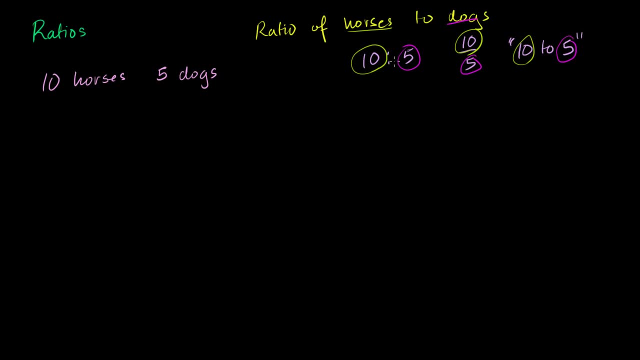 number of dogs. that's the number of dogs, or that's the number of dogs. These are all just expressions that are comparing two quantities. Now I just said I have 10 horses for every 5 dogs. But what does that mean? 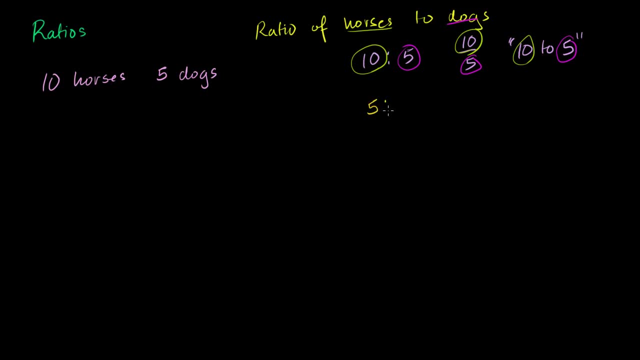 That means I have 5 horses for every 1 dog. Sorry, not 5 horses for every 1 dog. That means I have 2 horses for every 1 dog. If for 5 dogs I have 10, that means for every 1 of these. 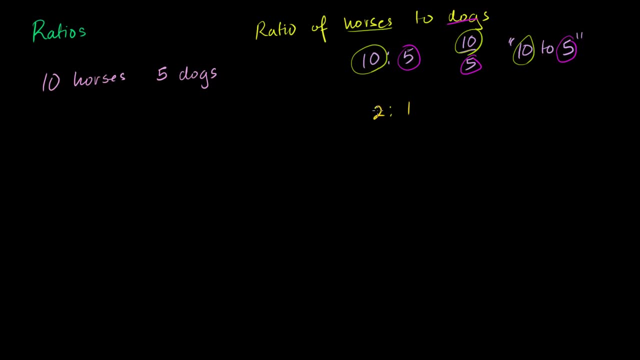 dogs. there are 2 horses For every 1 of these dogs. there are 2 horses. For every 2 of these horses there's 1 dog. And I just kind of reasoned, I reasoned through that. So this is: I have 2 horses for every 1 dog. 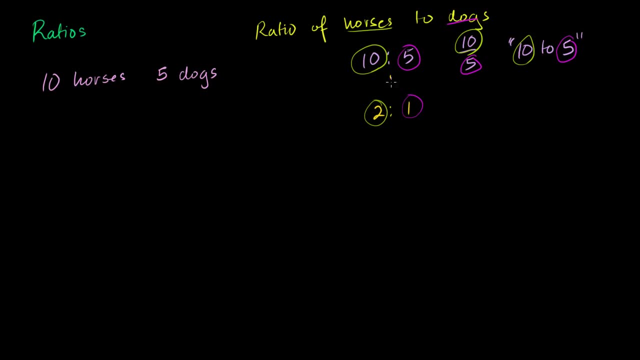 But how do you get there? How do you get from 10 to 5, to 2 to 1? Well, you can think of what's the biggest number that divides into both of these numbers. What's their greatest common divisor? I have a whole video on that. 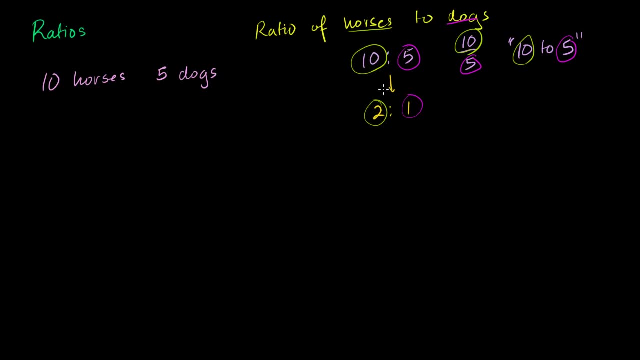 But the biggest number that divides into both of these guys is 5.. So you divide both of them by 5, and you can kind of get this ratio into a reduced form, And if I write it here it would be the same thing as 2. 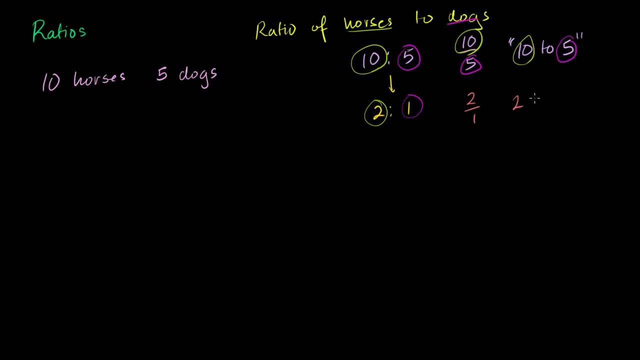 to 1 or 2 to 1.. And so what's interesting about ratios? it isn't literally, or doesn't always have to be literally, the number of horses and the numbers of dogs you have. What a ratio tells you is: how many horses do I have for? 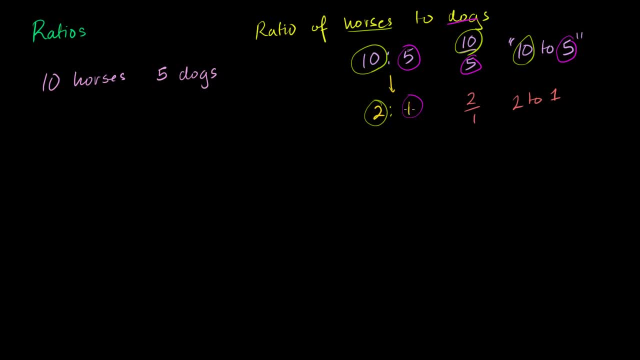 every dog, or how many dogs do I have for every horse? Now, just to make things clear, what if someone asked me: what is the ratio of? What is the ratio of dogs to horses? So what's the difference in these two statements? 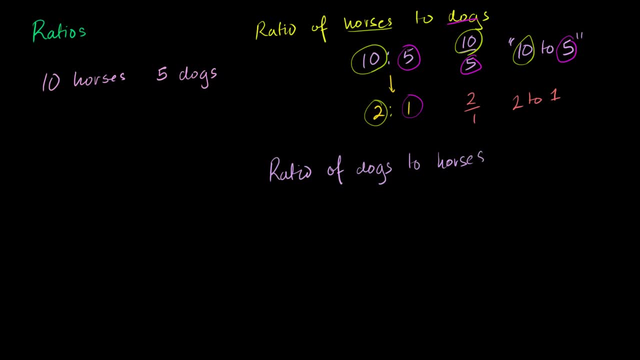 Here I said horses to dogs, Here I'm saying dogs to horses. So, since I've switched the ratio, what I'm looking for? I'm looking for the ratio of dogs to horses. I've switched the numbers, So dogs for every 5 dogs, I have 10 horses. 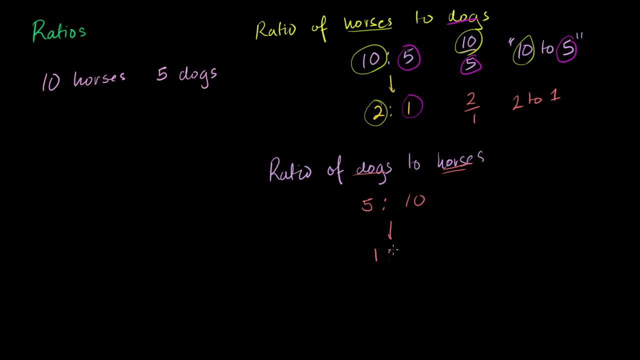 Or if I divide both of these by 5, for every 1 dog, I have 10 horses. I have 5 horses. So the ratio of dogs to horses is 5 to 10, or 1 to 5,, or you. 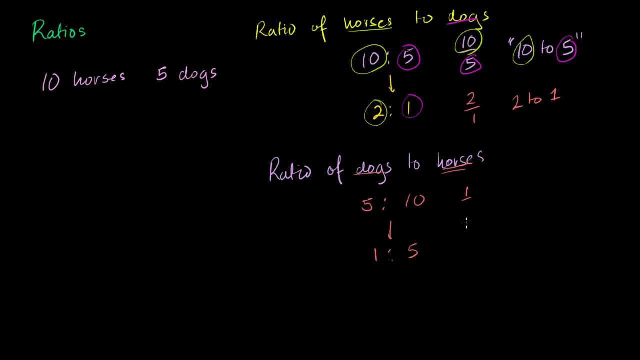 could write it this way. Let me write it down here: 1 to 5, or I could write 1 to 5. And the general convention. this wouldn't be necessarily incorrect, That's not wrong, but the general convention is to get. 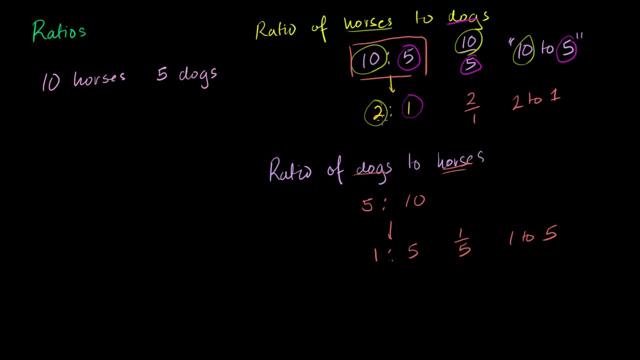 your ratio or your fraction, if you want to call it that, into the simplest form or into this reduced form, right there. So let's just do a couple of other examples. Let's say I have 20 apples. Let's say I have 40 oranges. 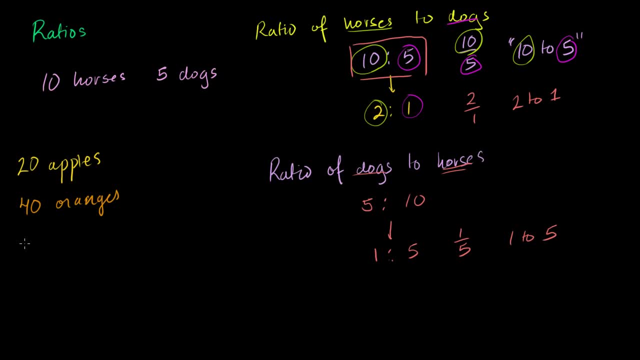 And let's say that I have, I don't know. let's say I have 60 strawberries, Strawberries, Strawberries. Now what is the ratio of apples to oranges to strawberries? I could write it like this: I could write what is the ratio of. I'll write it like: 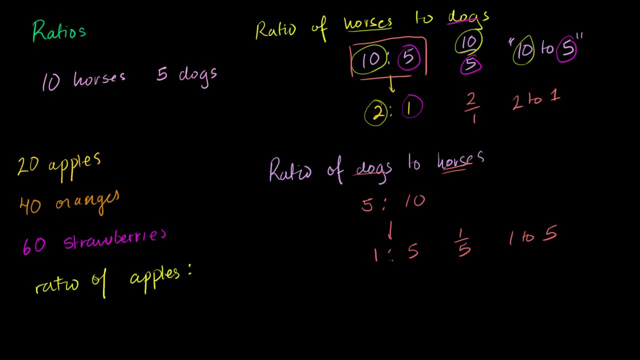 this: apples to oranges to strawberries. Well, I could start off by literally saying: well, for 60 strawberries, for every 60 strawberries, For every 60 strawberries, I have 40 oranges and I have 20 apples, And this would be legitimate. 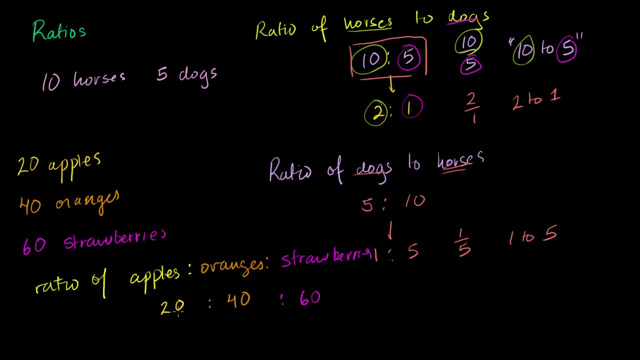 You could say the ratio of apples to oranges to strawberry are 20 to 40, sorry, 20 to 40 to 60. And that wouldn't be wrong, but we saw before we could put it into reduced form. So think of what's the largest number that divides. 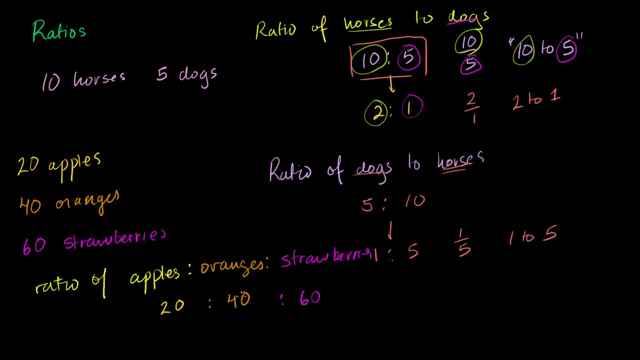 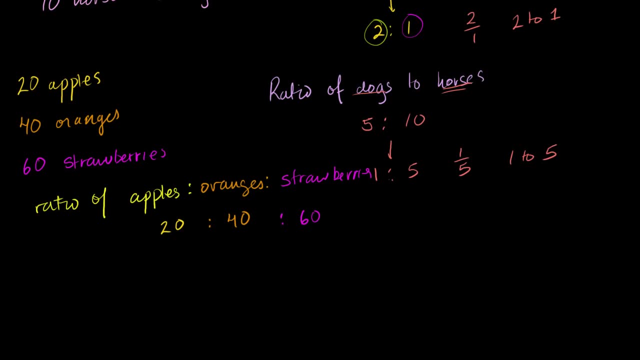 into all three of these. We can't just do it into two of these now, because now my ratio has three actual quantities. Well, the largest number that divides into all of these guys is 20.. So if we divide all of them by 20, we can then say for every: 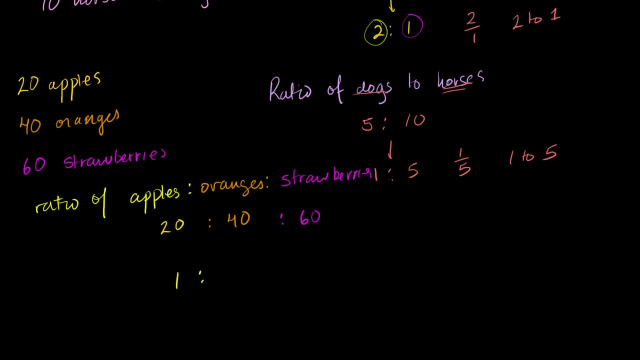 one apple I now have. if you divide this guy by 20, I have two oranges and I have three strawberries. So the ratio of apples to oranges to strawberries is 1 to 2 to 3. And I got that in every case by just 20.. 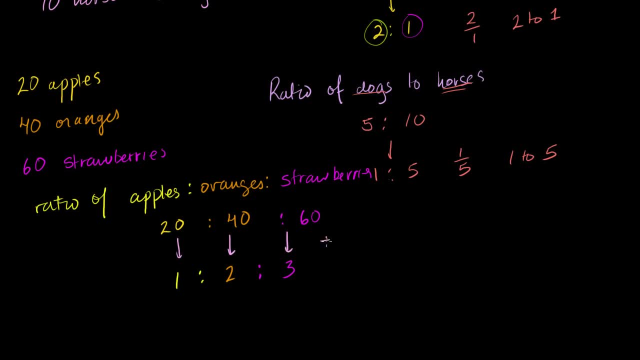 I'm just dividing these guys all by 20.. I divided by 20.. I think you get the general idea. If someone were to ask you what's the ratio of, let me just write it down because it never hurts to have a little. 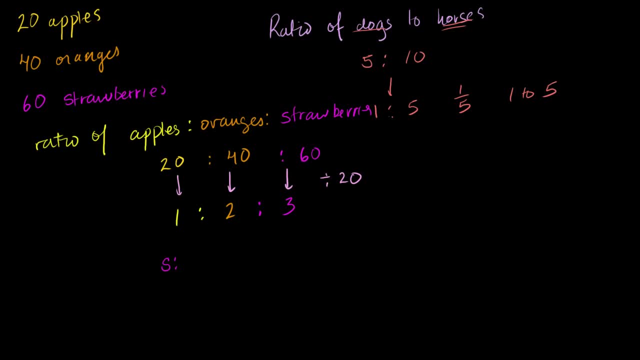 bit more clarification. If someone wanted to know the ratio of strawberries to oranges, let me get into my orange color: Strawberries to oranges to apples. I thought I was going to do that in yellow. What is this ratio going to be? For every three strawberries, I have two oranges and I have 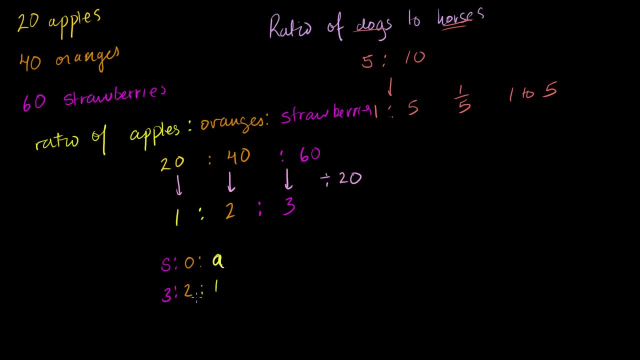 one apple. So then it would be 3 to 2 to 1.. The general idea is, whatever order someone asks you for the different items, the ratio is going to be in that same exact order. Now, in all of the examples so far, I gave you the quantity. 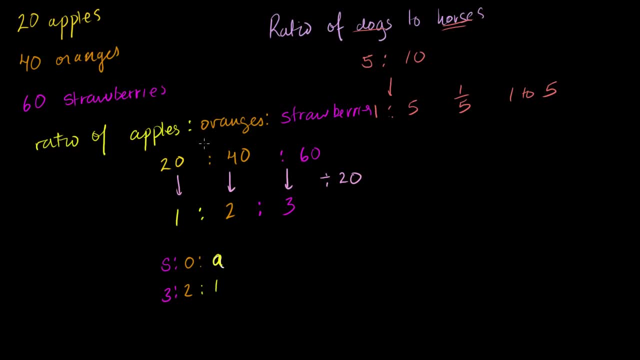 of things we had and we figured out the ratio. What if it went the other way? What if I told you a ratio? What if I said the ratio of boys to girls in a classroom is: let's say, the ratio of boys to girls is 2 to 3, which I could? 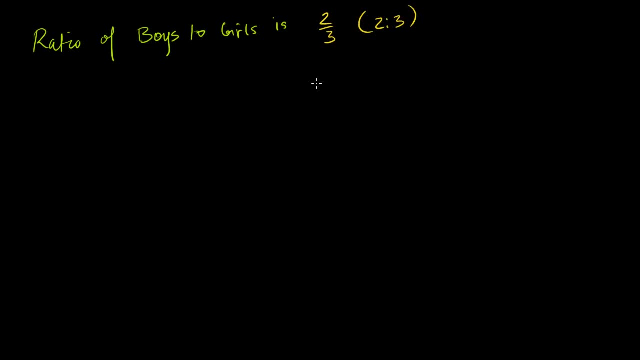 have also written as 2 to 3, just like that. So for every two boys I have three girls, Or for every three girls I have two boys. OK, OK, OK. And let's say that there are 40 students in the classroom. 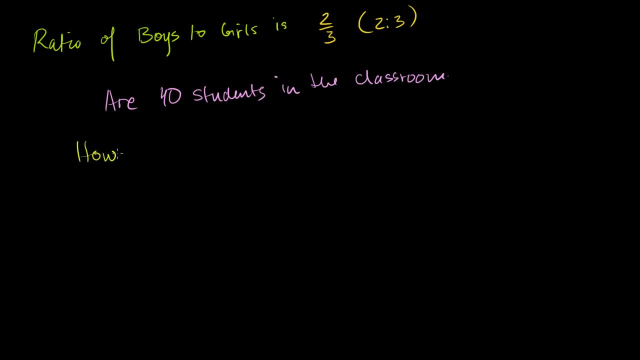 And then someone were to ask you how many girls are there, How many girls are in the classroom. So this seems a little bit more convoluted than what we did before. We know the total number of students, we know the ratio. 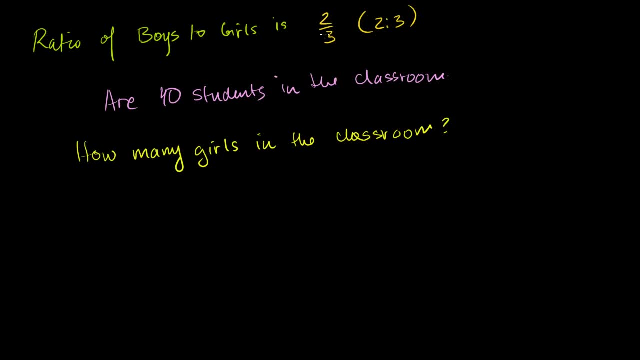 but how many girls are in the room? So let's think about it this way: The fact that the ratio of boys to girls- I'll write it like this: boys, maybe I'll be stereotypical with the colors- the ratio of boys to girls is equal to 2 to 3.. 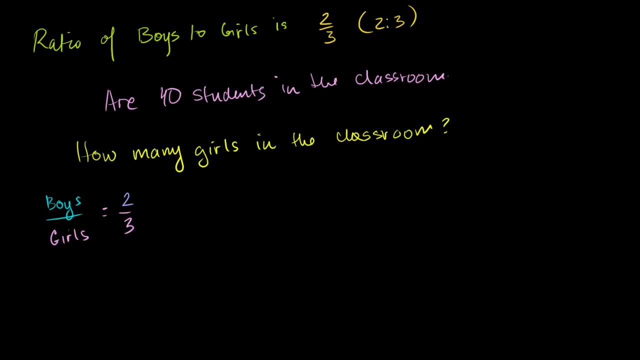 Hate to be so stereotypical, but it doesn't hurt. 2 to 3.. The ratio of boys to girls is 2 to 3, so this is: for every three girls, There's two boys. For every two boys, there's three girls. 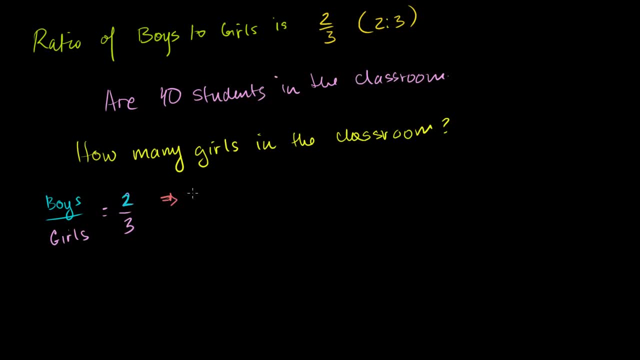 But what does it also say? It also says: for every five students, there are what? There are two boys and three girls. There are two boys and three girls. Now, why is this statement helpful? Well, how many groups of five students do I have? 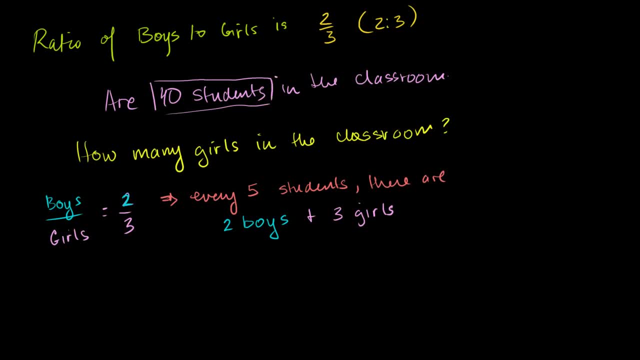 I have 40 students in my class. right there, I have 40 students in my class, And for every five students there are two boys and three girls. so how many groups of five students do I have? So I have a total of 40 students. 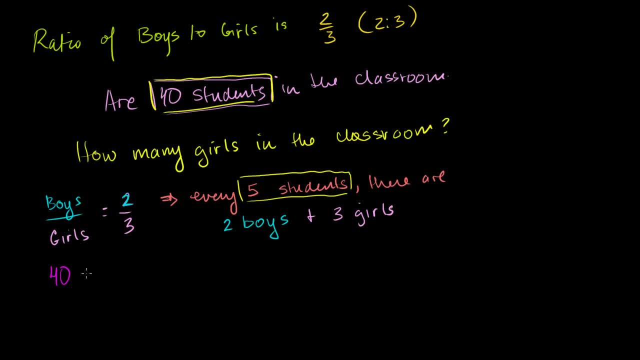 Let me do it in this purple color. I have 40 students, Five students per group, And I figured out that group just by looking at the ratio. For every five students, I have two boys and three girls. So how many groups of five students do I have? 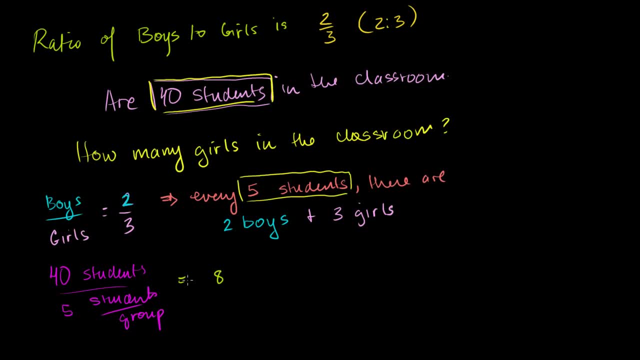 So that means that I have eight groups, 40 divided by 5.. I have eight groups of five students. Now we're wondering how many girls there are. So each group is going to have three girls. Each group has three girls, So each group has three girls. 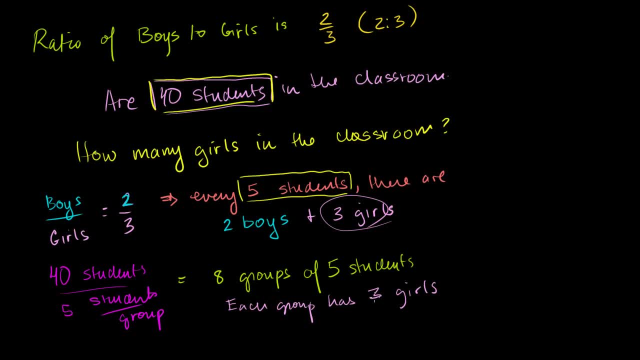 So how many girls do I have? I have eight groups. Each of them have three girls, So I have eight groups. times three girls per group is equal to 24 girls, 24 girls in the classroom, And you could do the same exercise with boys. 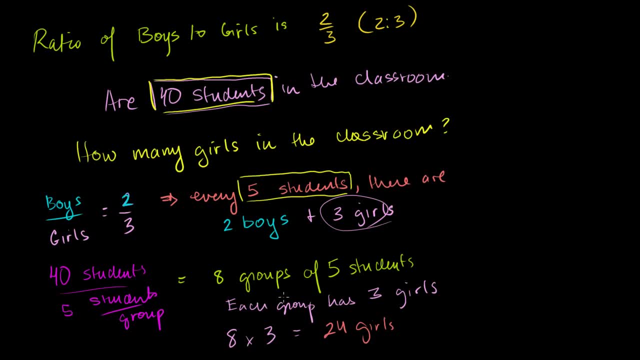 How many boys are there? There's a couple of ways you could do it. You could say: well, for every group there are two boys. There's eight groups, There's 16 boys. Or you could say: look, there's 40 students. 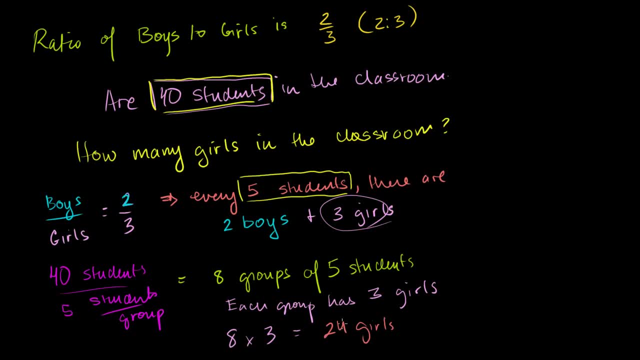 24 of them are girls. 40 minus 24 is 16.. So either way you could get to 16 boys And if you want to think of a kind of a fast way to do it and it would be identical, you'd say: look, 2 plus 3 is. 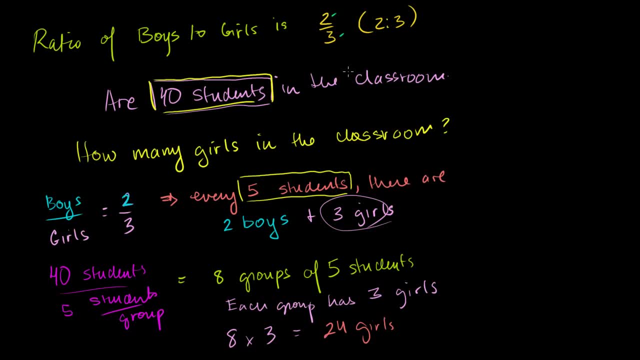 5, so for every five students, two boys, three girls. How many groups? How many groups are there? You say 40 divided by 5 is equal to eight groups. Every group has three girls. So you do: 8 times 3 is equal to 24 girls. 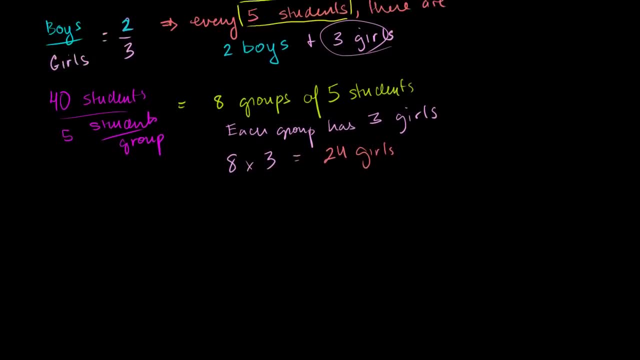 Let's do one that's a little bit harder than that. A little bit harder than that. Let's do one where I say that the ratio of- let's say- let's go back to the farm example- The ratio of sheep- I'll do sheep in white- the ratio of 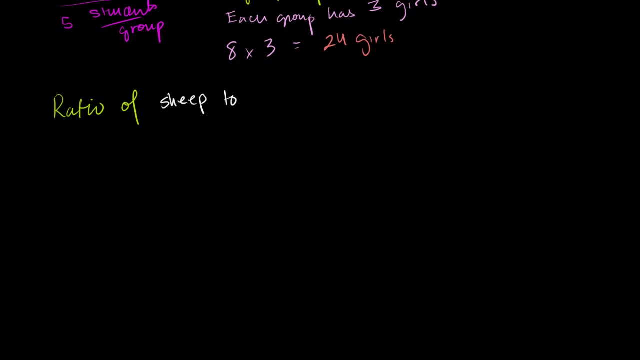 sheep to I don't know, chickens to chickens to I don't know what's another farm animal- to pigs. The ratio of sheep to chicken to pigs- maybe I should just say chicken right there. The ratio of sheep to chicken to pigs or chickens, I should. 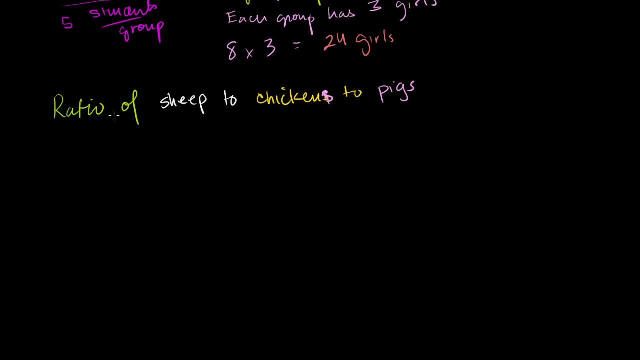 say, chickens Is. Let's say the ratio is 2 to 5,, 2 to 10.. And notice, I can't reduce this anymore. There's no number that divides into all of these. So this is the ratio of sheep to chickens to pigs. 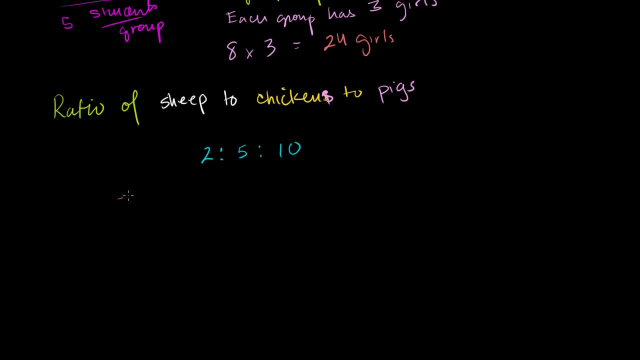 And let's say that I have a total of 51 animals. So I have a total of 51 animals And I want to know what's the ratio of sheep to chickens to pigs And I want to know how many chickens do I have?